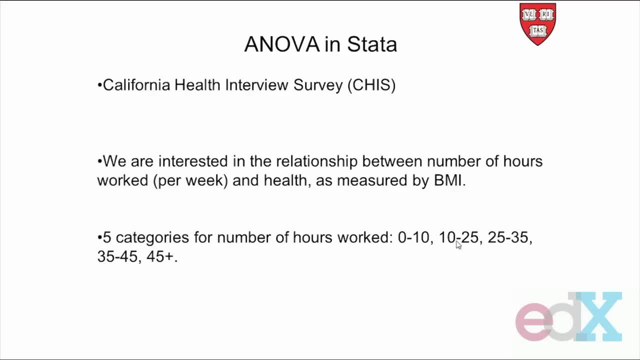 And this data is freely available to the public on their website, wwwchisuclaedu. So for this lab we're going to use a sample of 500 adults And suppose we are interested in the relationship between number of hours worked per week and health as measured by BMI. 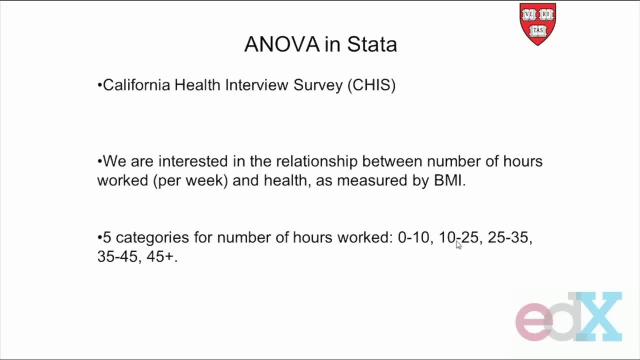 So we're going to break number of hours worked. We're going to break that up into five categories: 0 to 10,. 10 to 25.. 25 to 25.. 25 to 25.. 25 to 35.. 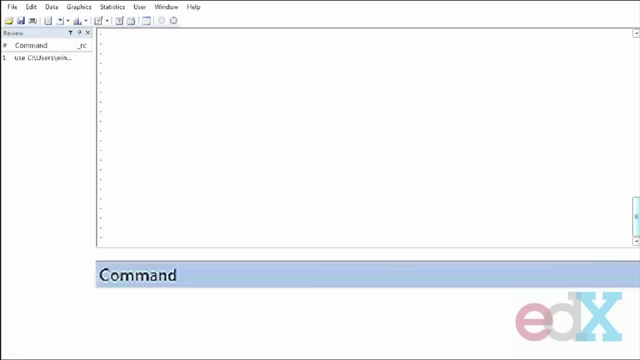 35 to 45. And 45 plus. So if you would open up the chisanovadta dataset in Stata, the first thing we're going to do is we're going to find out how many people are in each category, in each work category. 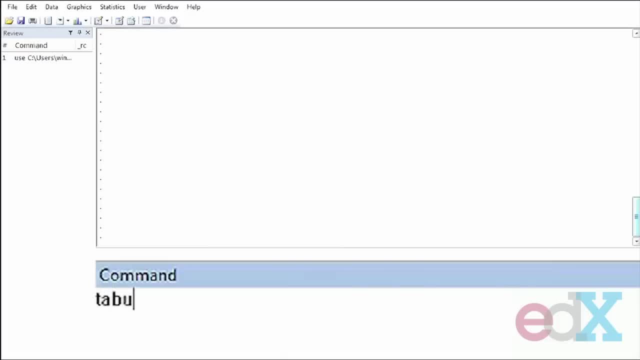 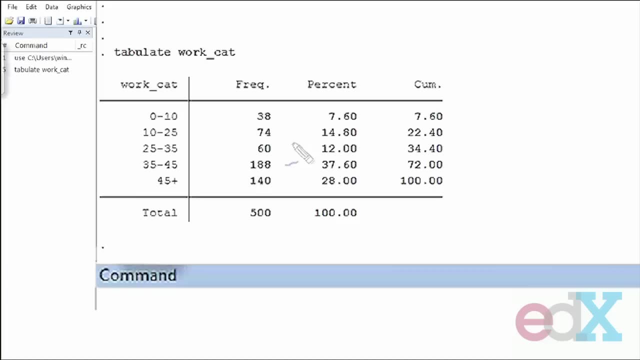 So to do that, simply type in tabulate work category And we can see the frequency now of each work category group. So for instance, the group with the most observations is the 35 to 45 group. So suppose now we wish to run an ANOVA. 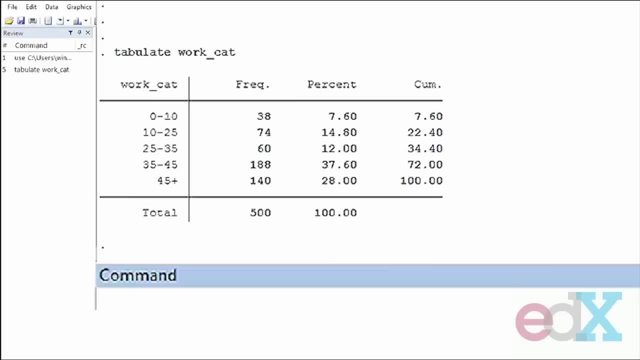 Now are the assumptions for ANOVA met. So the one assumption of independent groups. we have that here. So the next two assumptions are that the data must be normally distributed with equal variance. So to check this assumption, we're going to create a histogram of BMI by work category. 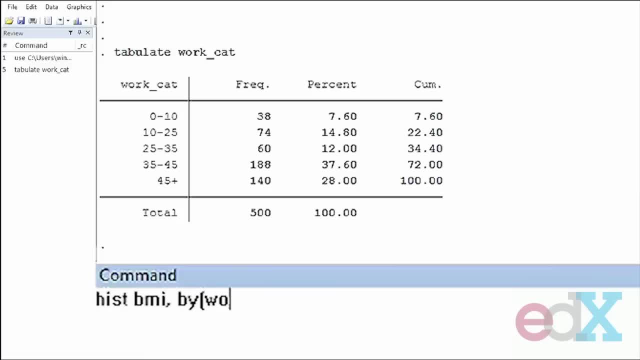 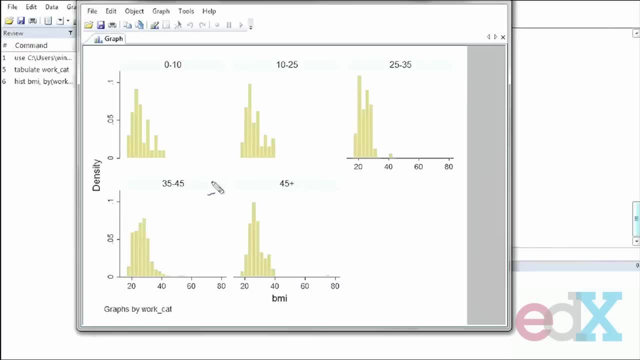 And to do that, type in the following command: Histogram of BMI by work category. And we can see from these histograms that the data are approximately normally distributed. They seem to have equal variance. There's nothing really strange going on, So it's safe to assume that the data, that the assumptions for ANOVA are met. 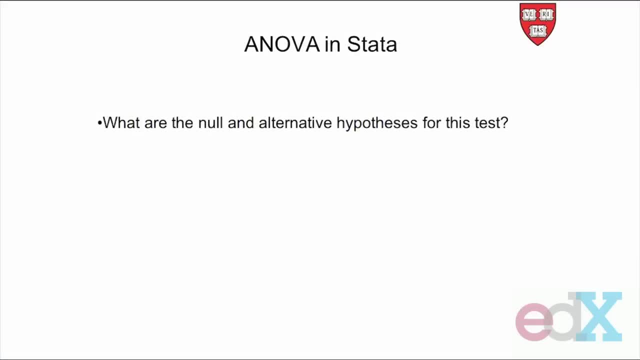 So now we want to run an ANOVA, But the first thing we want to state is our null and alternative hypothesis. So what our null hypothesis is is that the mean for the first category of work group, the mean of BMI, is equal to the second. 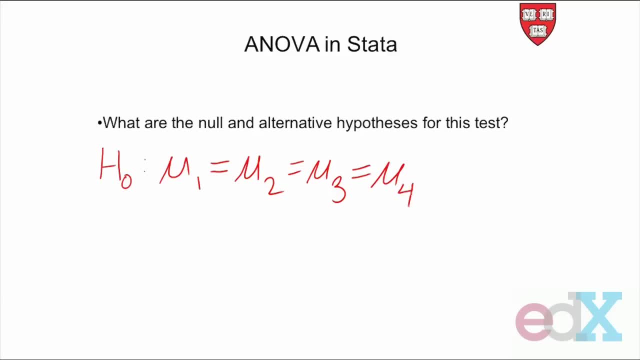 It's equal to the third, It's equal to the fourth, It's equal to the fifth. So the means of BMI in each work category are equal, And the alternative, we can just say not so. So what do we mean by that? 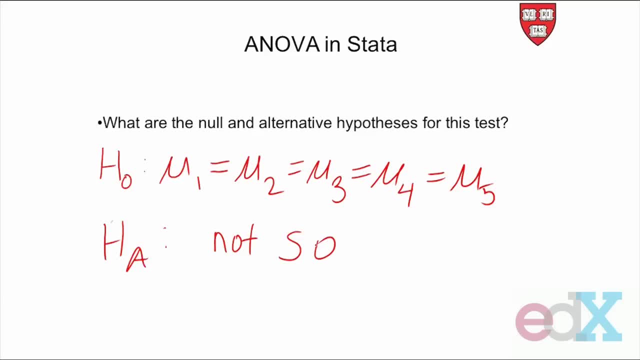 We mean there's at least one not equal sign somewhere in that null hypothesis. We don't know if they're all not equal. We don't know if only group four and group five are not equal. But we're just saying, we don't know which ones are equal, but we know that they're not all equal. 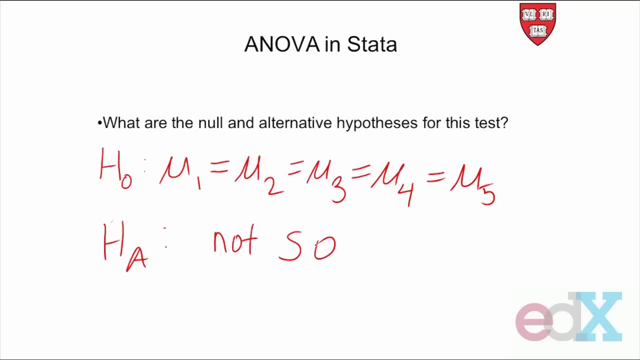 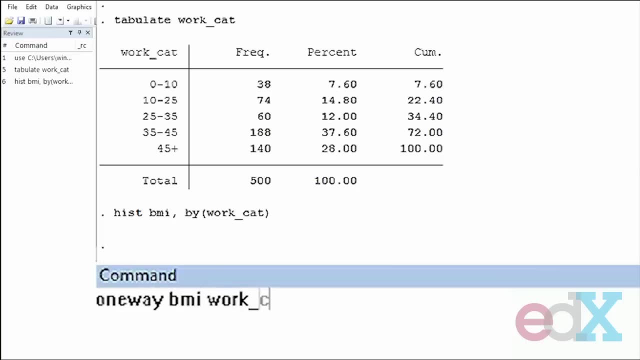 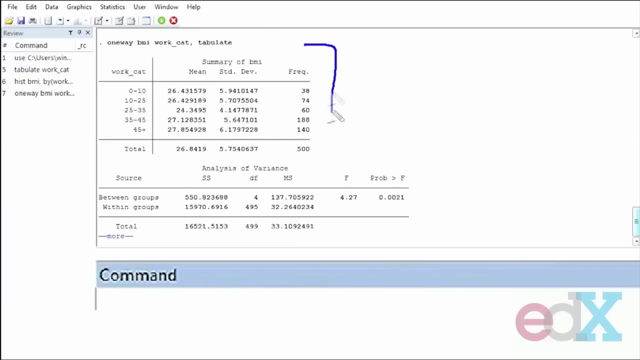 So that's our alternative hypothesis. So now we're going to go back to Stata And now we're going to run an ANOVA And to do that type in the following command: Now hit enter, And so the first thing we see is a summary of BMI. this table up here. 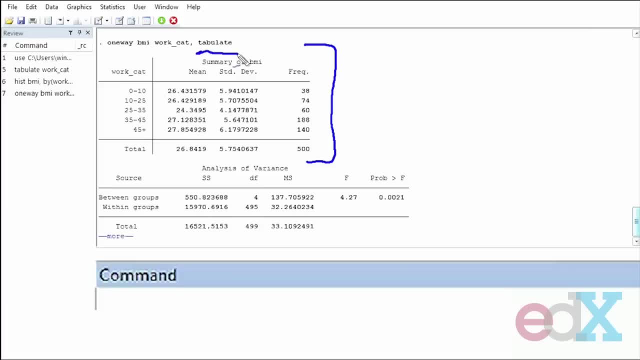 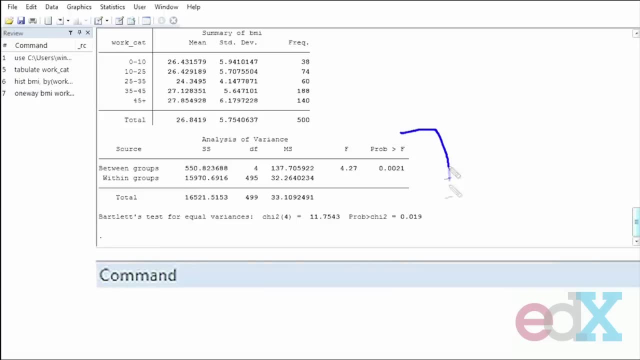 And we get this table, And we're going to do that by using the tabulate option. So what this will show us is the mean and standard deviation for each category, And then down here we have our analysis of variance table. So the first thing we want to find out what's our test statistic. 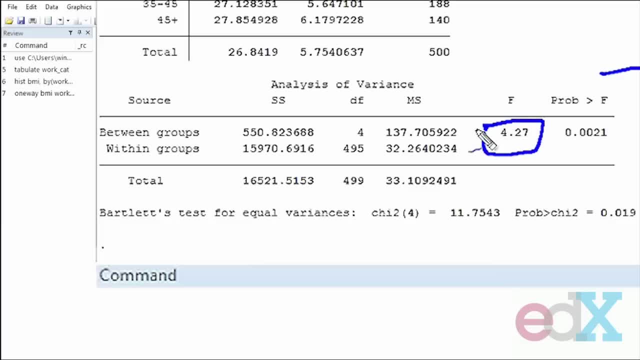 And our test statistic is this F value? right here, Our test statistic is 4.27.. Now, what are our degrees of freedom? Now we know that the F distribution is indexed by two degrees of freedom, And so what we have here is the numerator has degrees of freedom four. 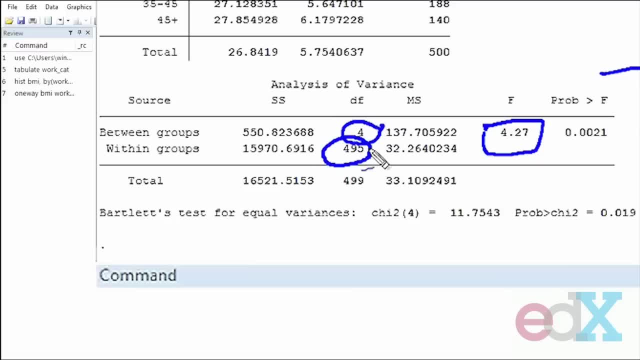 And the denominator has degrees of freedom: four, ninety-five. So those are our degrees of freedom. Next thing we want to find out is what's our P value? And we can see that our P value right here is 0.0021.. So let's run this. let's say we choose an alpha of 0.05.. 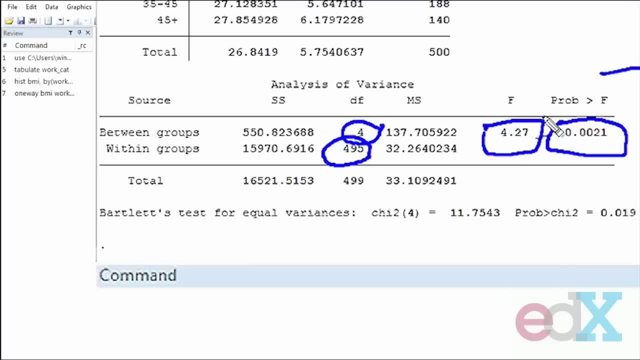 If we choose an alpha of 0.05, then with this P value we have rejected the null hypothesis. So what does that mean? That means that we have evidence that at least one pair of means are not equal, And the natural question that arises from that is: well, which pair of means are not equal? 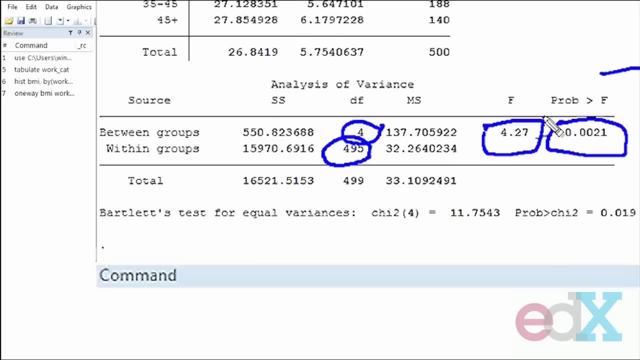 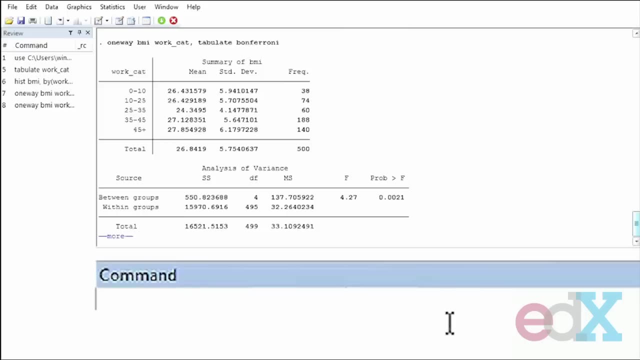 And to do that we can perform all possible pairwise comparisons using the Bonferroni correction And to do that, type in the following command. So you'll notice a new option we added to the one-way command. We added this: This is the Bonferroni option. 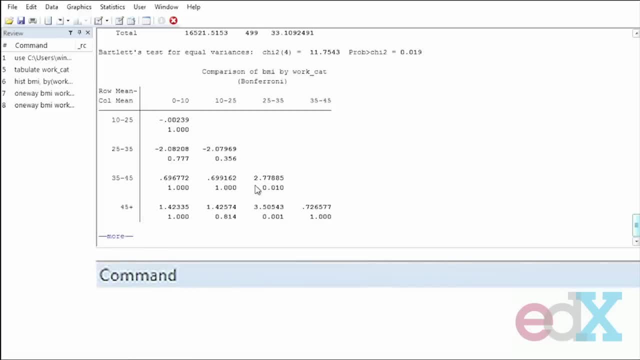 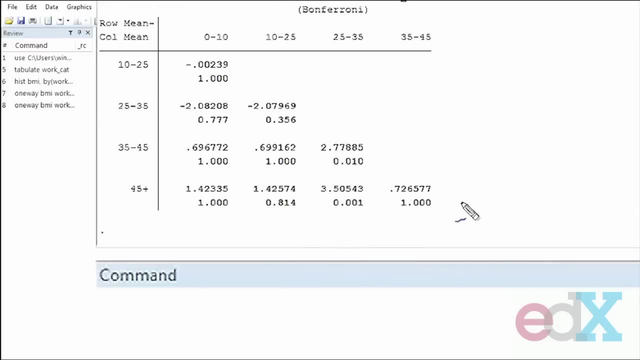 And what that does is that gives us this table down here. So now we have all pairwise comparisons. So what is this table? How do we interpret this table? So we have our categories up here: 0 to 10,, 10 to 25, and so on. 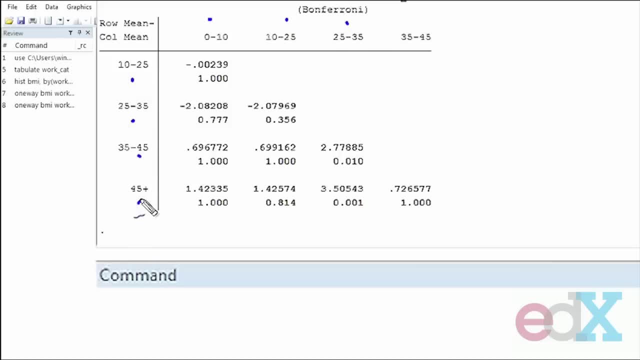 And then 10 to 25,, 25,, 35,, 35, to 45 and 45 plus, And so the first number is simply the row mean minus the column mean. So that's simply The mean of BMI for 10 to 25 minus the mean of BMI for the 0 to 10 category. 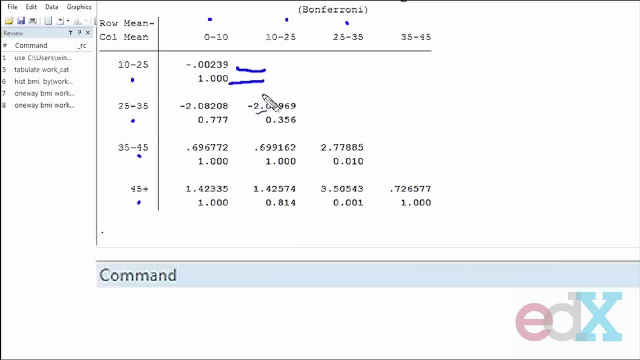 Now below: that is our p-value for the comparison. Now Stata is smart and Stata already adjusts this p-value to account for multiple comparisons. What we have to do is we have to compare these p-values to 0.05.. And if Stata- because Stata automatically adjusts the p-value for multiple comparisons- 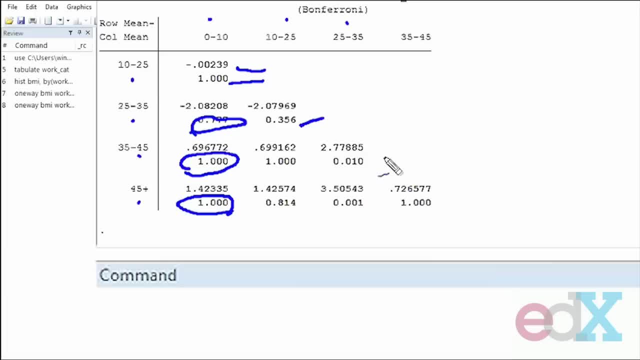 And if Stata didn't do that for us, We would have to compare these p-values to: 0.05 divided by 5, choose 2. Because that's the formula that we learned for multiple comparisons. So now we can see that there's two pairs of means that are not equal. 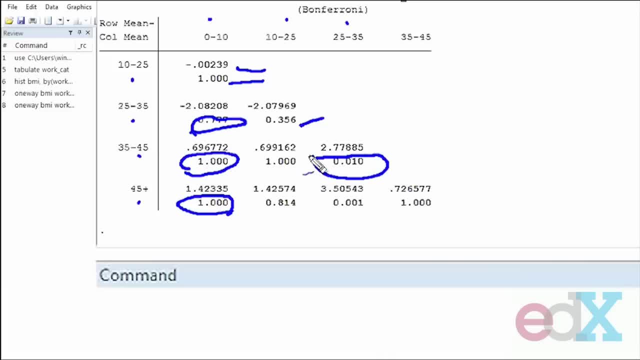 The 25 to 35 compared with the 35 to 45. That's a p-value of 0.01.. And the other one is the 25 to 35 and the 45 plus, And those two pairs of means are not equal. 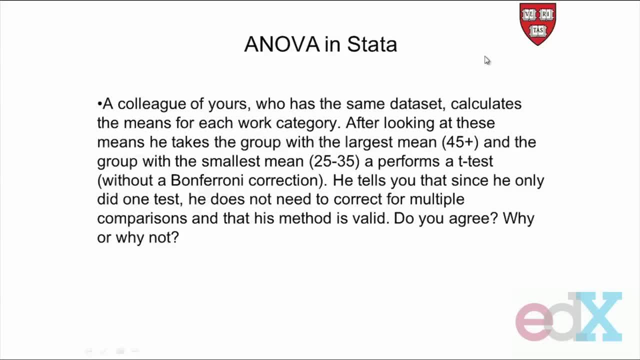 And that's how one would run an ANOVA in Stata. Now consider the following situation: A colleague of yours, who has the exact same data set, calculates the means of BMI for each work category And after looking at these means, he takes the group with the largest mean.